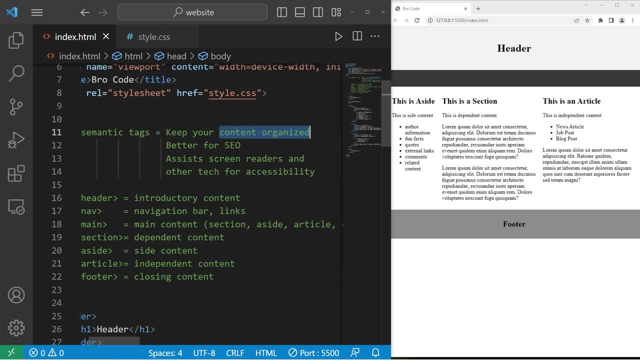 You'll want to use semantic tags because they keep your content organized, they're better for search engine optimization and they assist with screen readers and other technology for accessibility. So I've already written some HTML markup. I just want to describe this first. 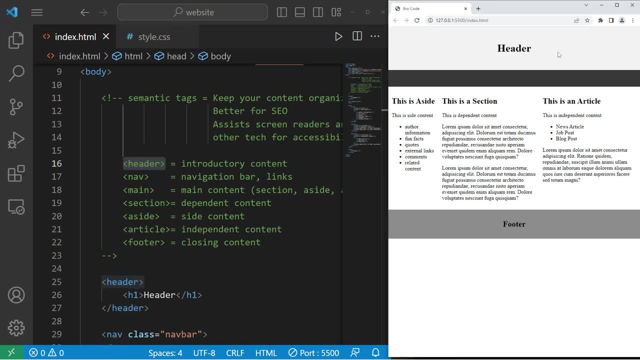 Headers are used for introductory content, such as a title, a logo or author information. Nav elements. they're used for navigation bars or other links. Sometimes you may find a set of navigation links at the bottom of your page, but having a navigation bar is fairly common. 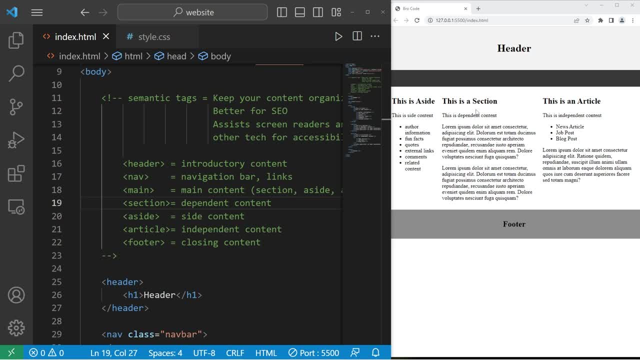 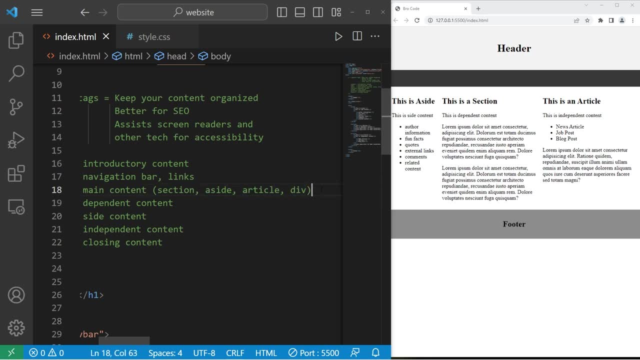 Now the main content, which is all of this. it can contain one of many sub-elements, such as sections, assignments and more Side elements, articles and generic div elements, So sections, which is what I've created here in the middle. this is for dependent content. 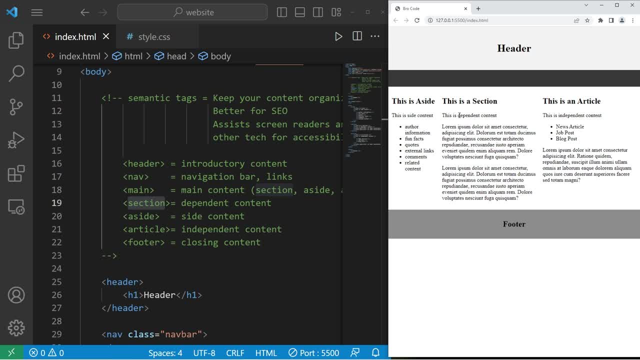 You would typically put anything you want within a section. It's typically used for dependent content. If I were to take this section out of the webpage then put it on another webpage, it might not necessarily make sense. Like what is it for? 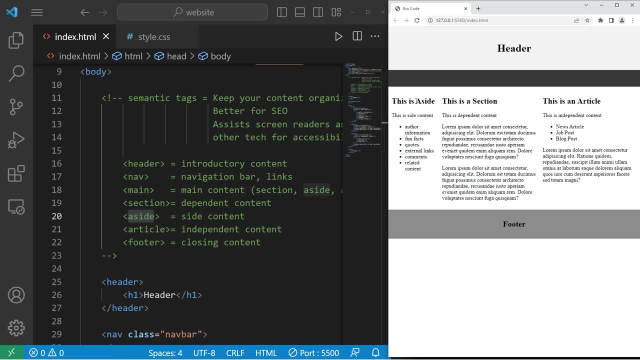 That's why it's dependent And a side element is meant for side content. This can include author information, fun facts, quotes, external links, comments or really any other related content that's related to a section, Now an article. this represents independent content. 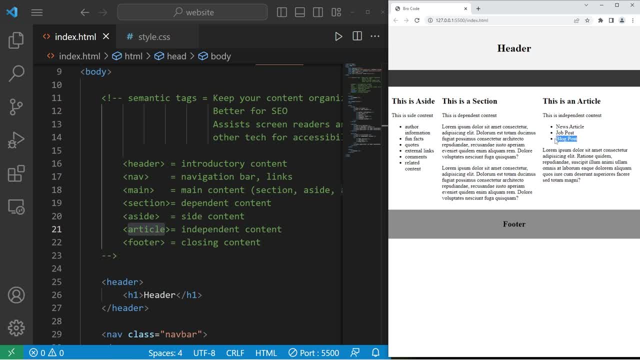 This could include news articles, job posts or blog posts. Articles are really similar to sections. With articles it's meant for independent content, For example, a news article. If I were to take this news article, cut it out and put it on a different website, 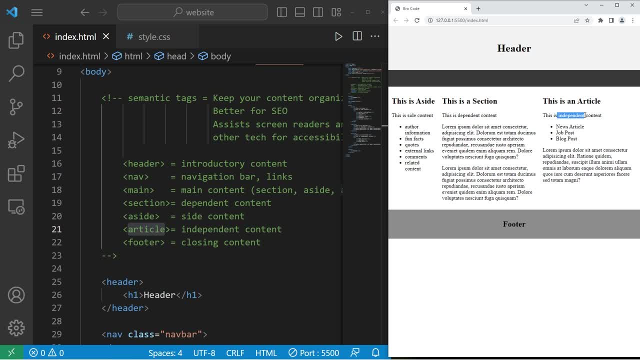 it would still make sense. It's independent content. It's not reliant on the context of the website, whereas in a section would be. And then, lastly, we have footers. A footer is for a closing content. This could include author information, copyright information and sometimes navigational links. 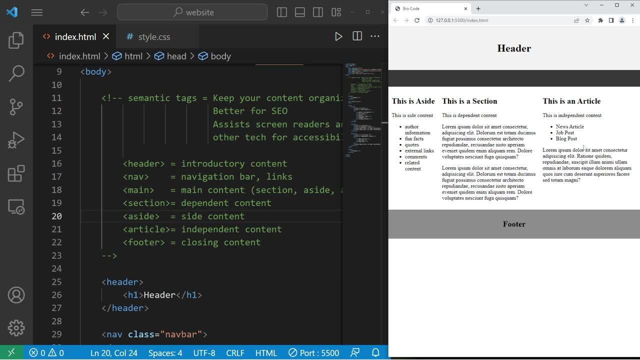 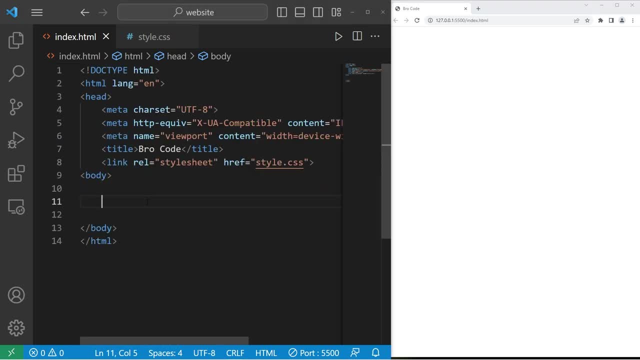 There's really no one-size-fits-all approach. Really, the design is up to you, but this is a really common format. Now that we know the basics, let's actually design this. Alright, so we will create our semantic elements. We have a header, a nav element, a main element and a footer element. 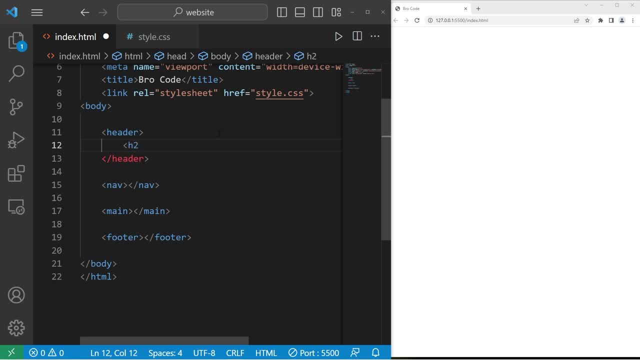 Within our header element. let's just add an h2 element that says header. So let's go to our style sheet. I'll take our header element. Let's change the background color. Background dash color. Let's pick a light gray color. 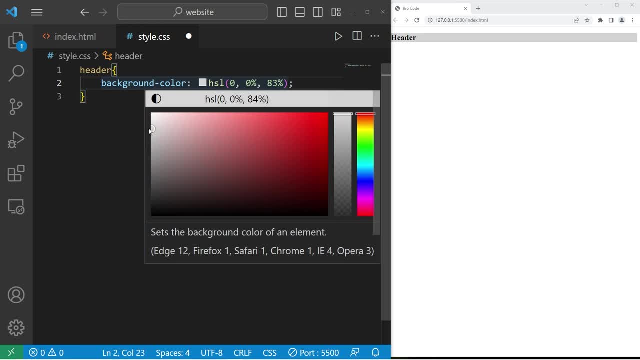 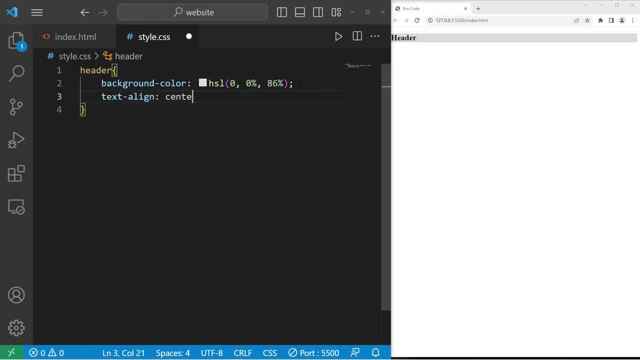 I'll use HSL values because I like them. 84 or 85 is good. Then let's text align center And add a little bit of padding: 25 pixels. Okay, let's work on our navigation bar. It's not going to be a fully functioning navigation bar. 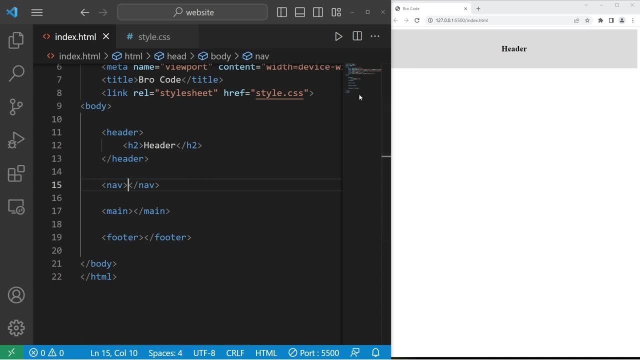 We've done that in a previous video. Let's just allocate some space for a navigation bar. It is common to have more than one navigation bar. If we're creating a navigation bar, we should set the class to be something like navbar, so it's descriptive. 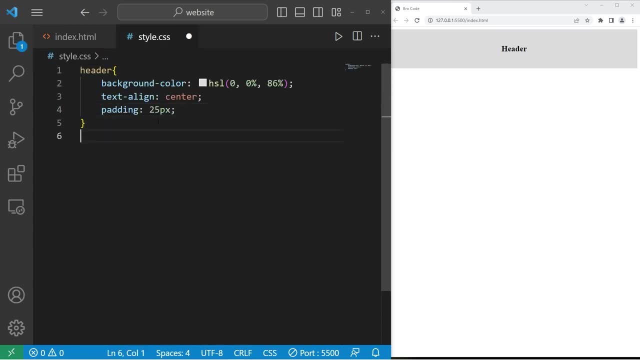 Let's go to our CSS style sheet. I will select our navbar class, then change the background color. Let's go with the darker color. I'll add some height, Height, 50 pixels, And that should be good. We're just allocating some space. 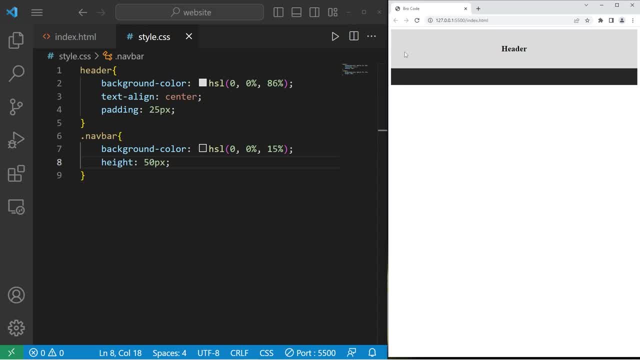 We're not creating a full navigation bar. There's a little bit of margin around the body of our document. I'm going to remove that by selecting our body element. Then set the margin to be zero or zero pixels. That should get rid of the margin. 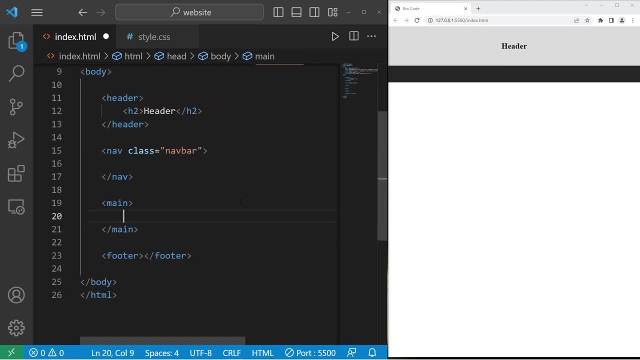 All right, then we have our main element. Our main element can include any combination of aside sections, articles or even just some generic div elements, But we won't be working with div in this video. Really, you can see any combination of aside section, article or div. 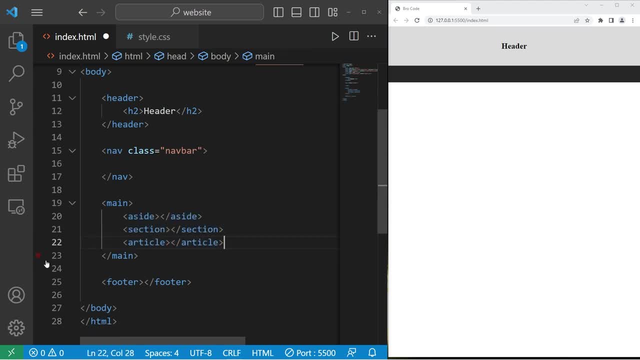 Or maybe even none of them. It's up to you. In this topic, we'll stick with one aside element, one section and one article. These elements are kind of like sub-elements within our main element. Our main element is going to be the main steak and potatoes of our web page. 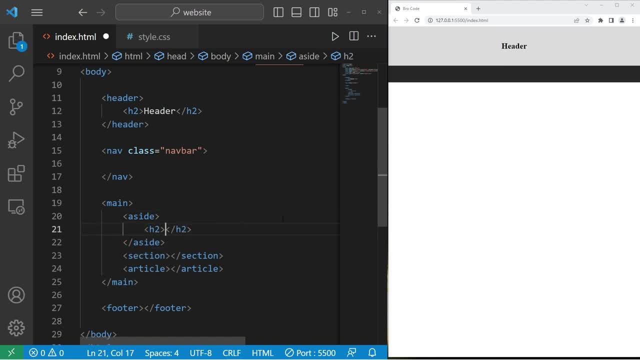 So, with our aside element, we're going to use our main element as our main element. I'll include an element for a header. This is a side. Let's do the same thing for section. This is a section, Then this is an article. 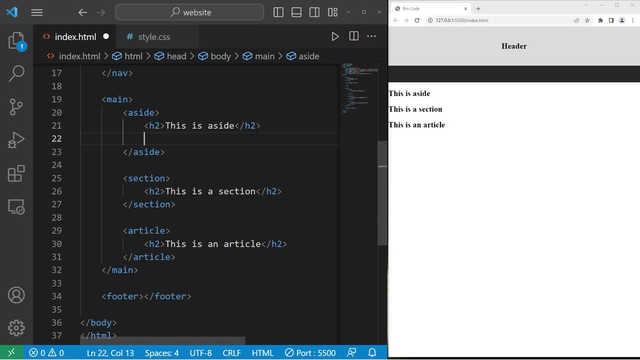 Let me separate these just so that they're easier to see. Just to take up some space, I'm going to create some sample paragraphs. Our side element We'll have one. Our section will have two paragraphs. I'm just copying and pasting. 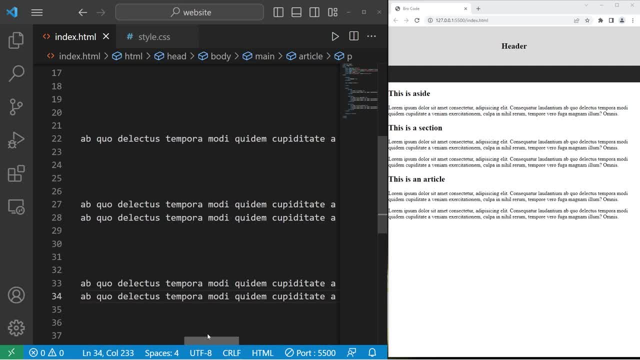 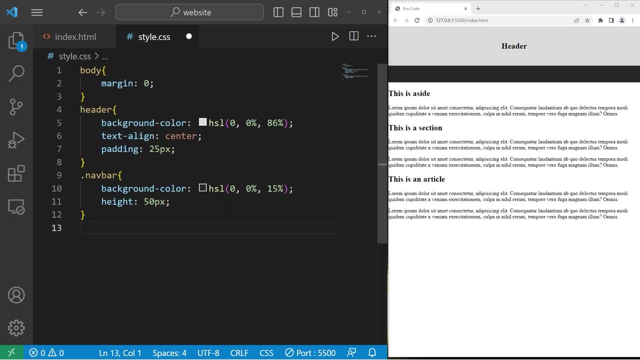 And our article will have two as well. I don't want this top to bottom layout. We can change that with some CSS properties, So let's work on our aside element first. With our aside element, I'll set the width to be 20% of the width of the web page. 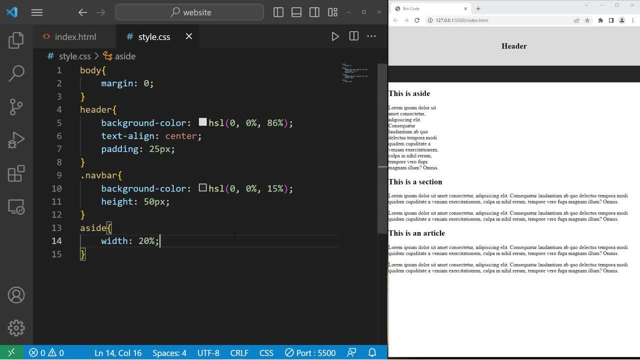 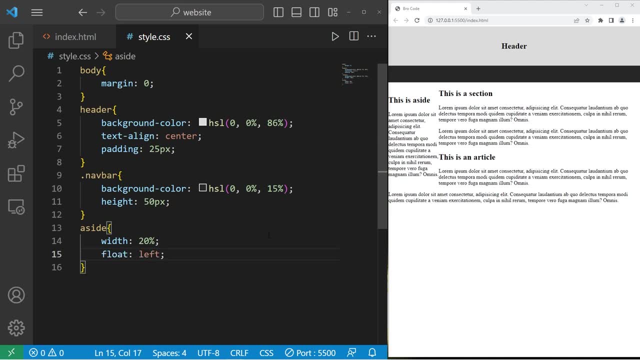 Our aside element only takes up 20% of the space. To have that space available, the following elements can float: We have to set the float property to be left then in this case, Alright, let's copy aside. Change aside to be section. 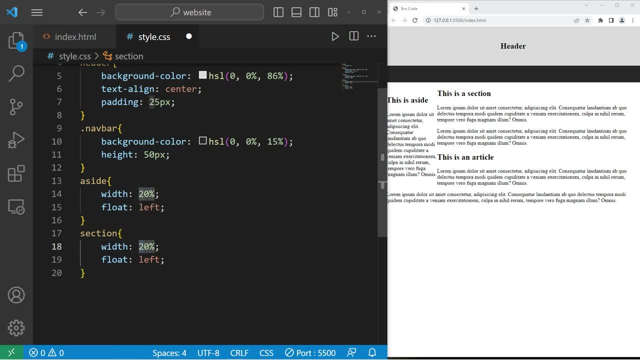 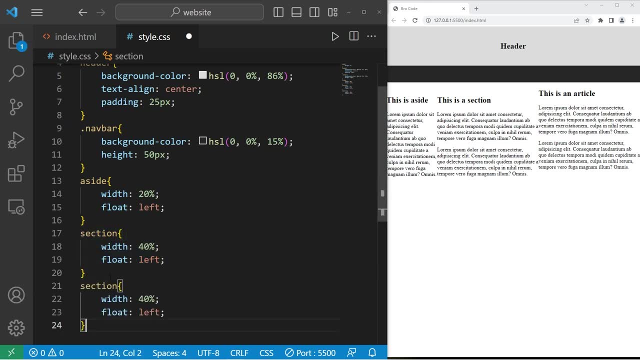 That's our next element. I'll set the width to be 40%. Then we have article Change section to article And the width will stay at 40%. These three elements make up our section. These three elements can all fit within the web page. 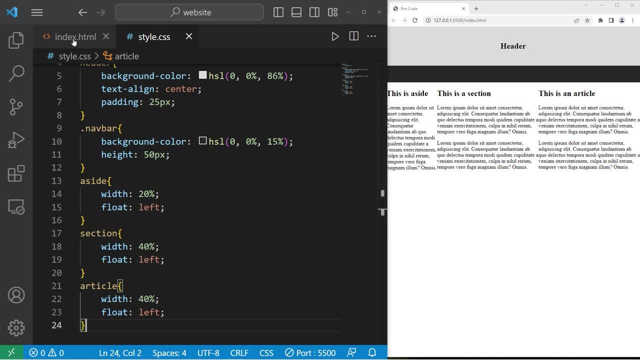 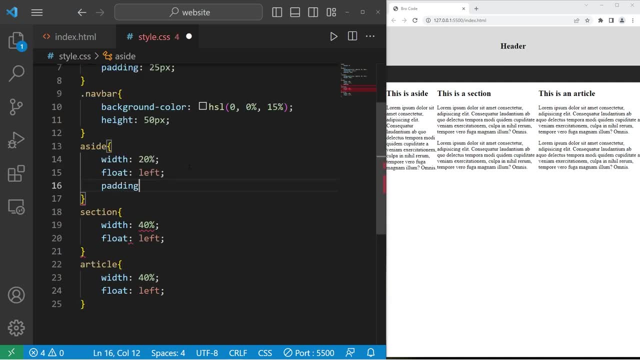 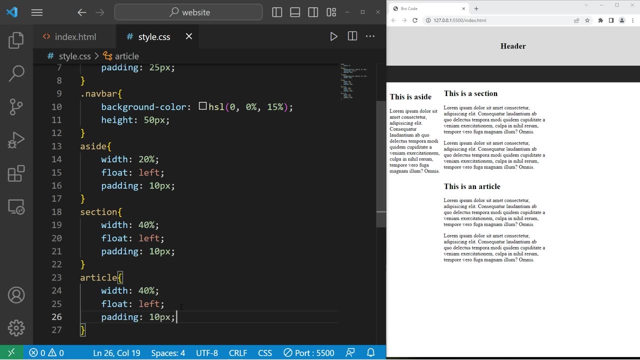 The total width is under 100%. We have our three elements within our main element, So if you would like to add a little bit of padding, this is what you're going to do. Let's add 10 pixels of padding to each of these elements. 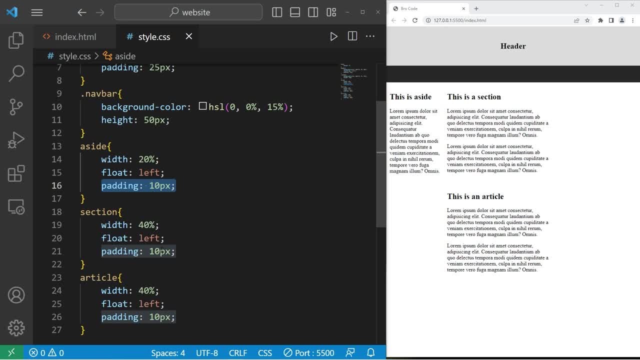 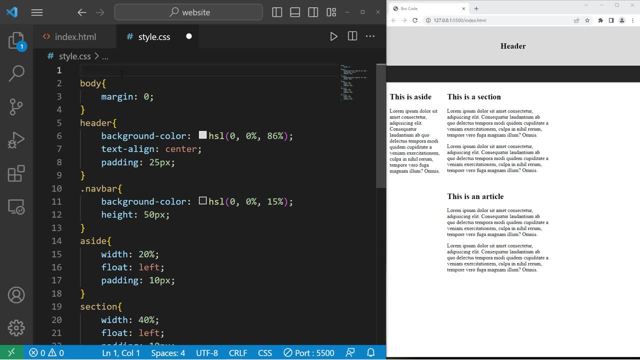 When we calculate the width, we don't take into account any padding. So one change we're going to make is that at the top of our CSS style sheet, we can select all elements with an asterisk, then a set of curly braces. 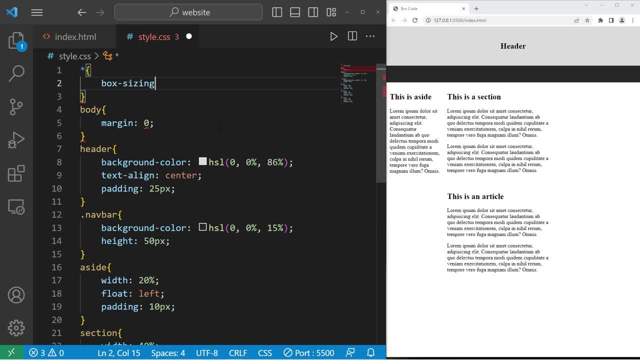 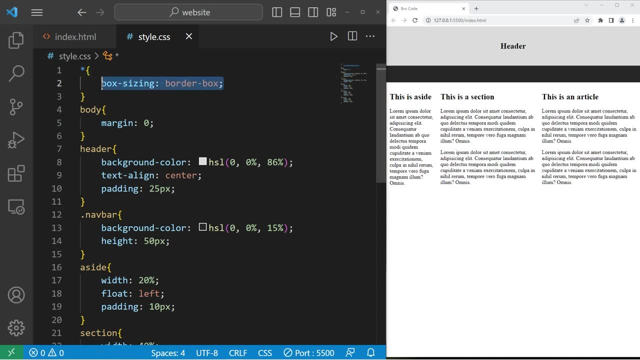 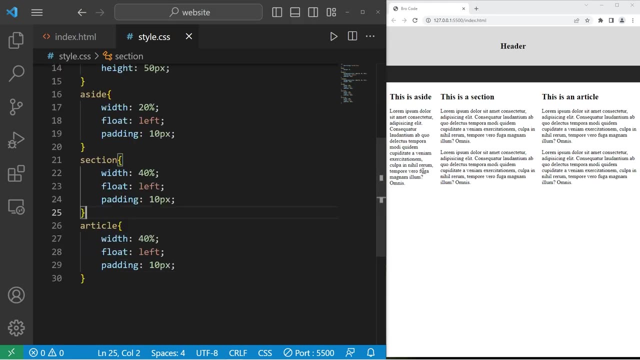 We will set the box sizing property to border dash box. What we're doing with this property is that when we calculate the width factor in the padding, All three elements should be lined up now. Alright, then, lastly, we have our footer.